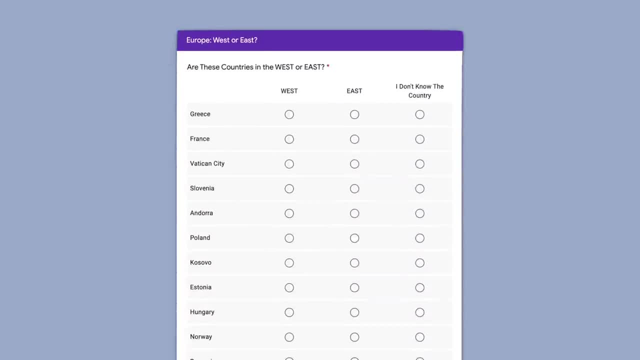 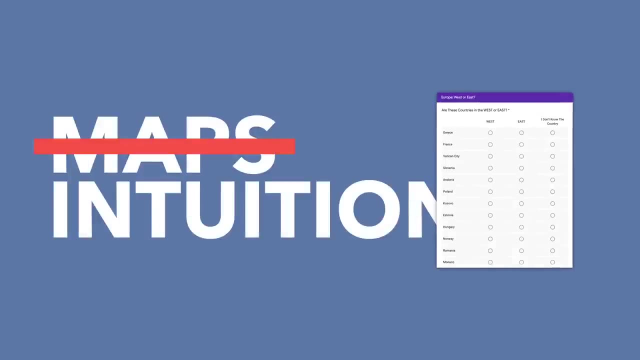 In one poll, we asked people if the nations were in the East or the West, without any geographical hints, with us explicitly telling them not to look at maps. In the other poll, though, we gave voters maps marking exactly the country they were assessing. 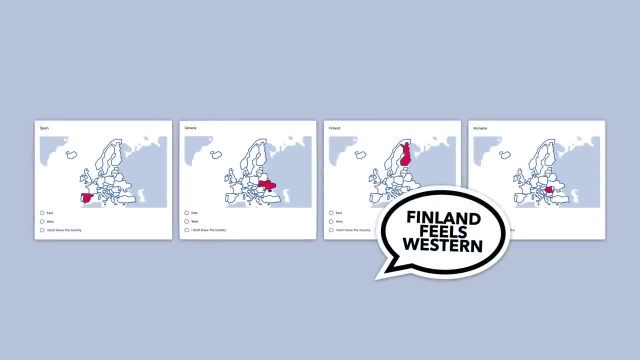 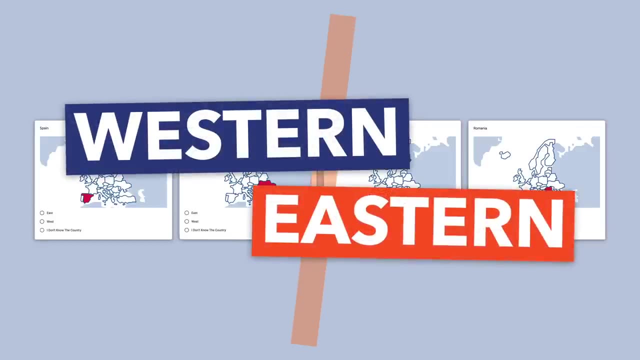 We did this as we were interested if knowing the exact geographical location of the countries would impact people's intuitions. Anyway, before we get into that data, let's draw the line. Some countries very clearly fell on one side of the line or the other. 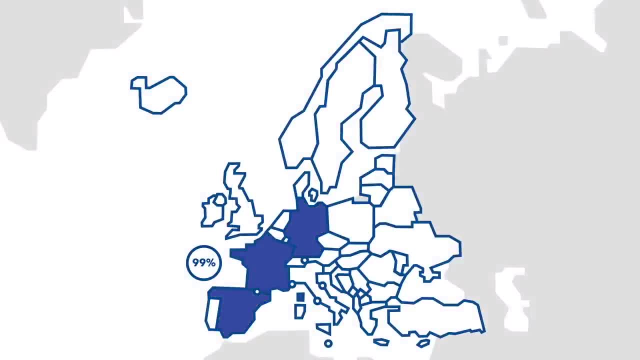 More than 99% of people put France, Spain, Germany, Italy, Ireland, Iceland, the UK, Denmark, Switzerland, the Netherlands, Belgium and Luxembourg in the West, And all of these other places had more than 90% West. 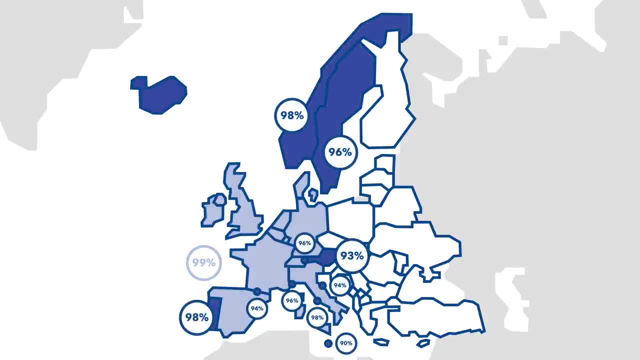 On the other side, though, it was a little less cut and dry, 13 countries were almost unanimously voted as Western, but only one country got more than 99% East: Belarus. Getting more than 90% East, though, we had Ukraine, Moldova, Bulgaria, Turkey, Romania, Serbia. 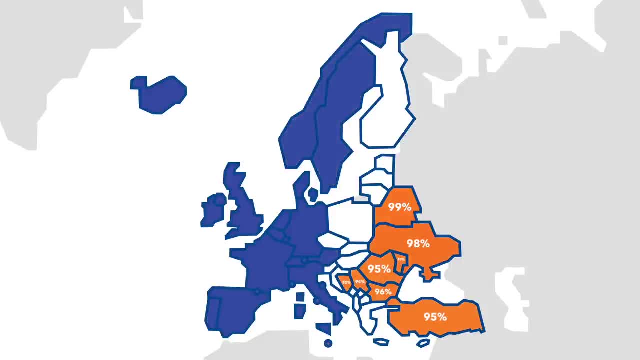 Bosnia and Herzegovina, Albania, North Macedonia and Kosovo. So we don't have a clear line of the two. We will do by the end of the video, but there is already a clear divide, despite the fact that we've only coloured where the audience was in at least 90% agreement. 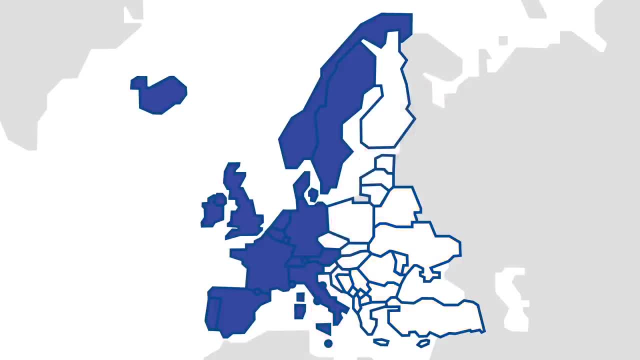 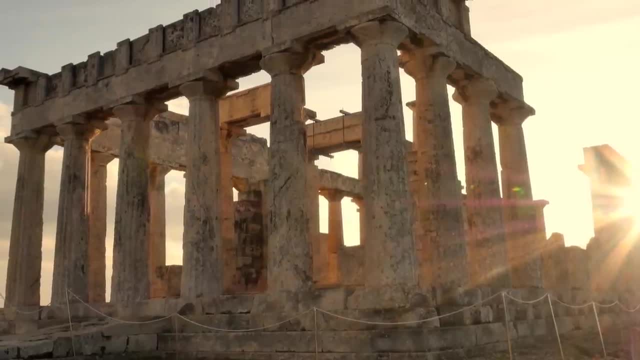 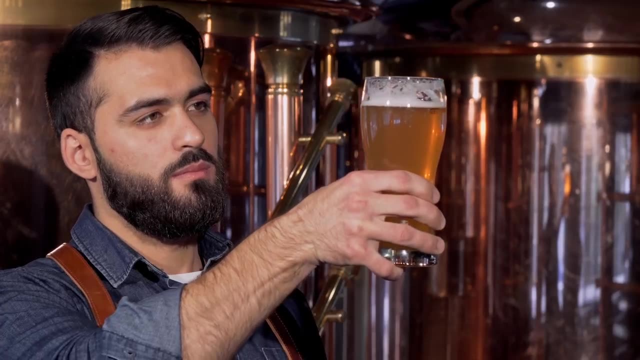 It's clear, geography is a factor here. I mean, those marked in the West are clearly in the West and vice versa. but it's not the only factor at play. History and culture are other fairly clear dividing lines with fairly different traditional cultural practices on each side of the continent. 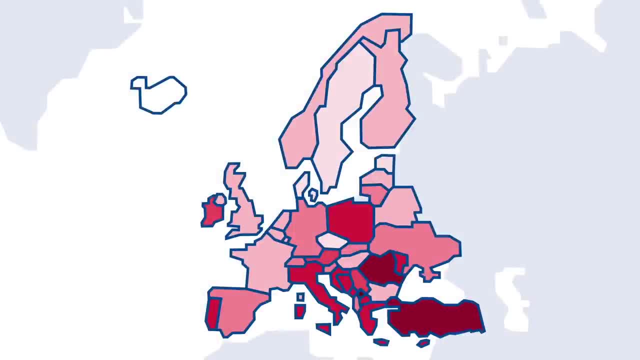 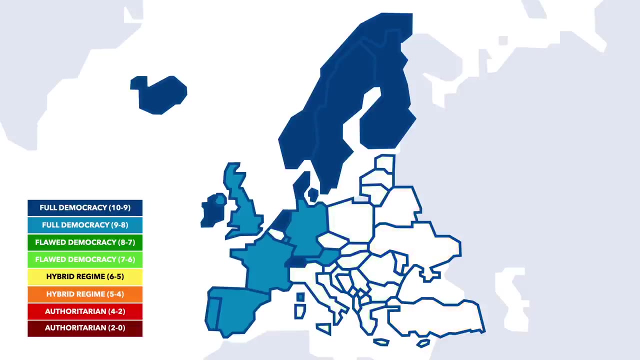 For example, when we look at the level of religiousness for each country, we can see that many, but not all, of the most religious countries fall on the Eastern side, geographically. It's even clearer when we look at democracy, though, with many of the stronger democracies falling on the Western side. 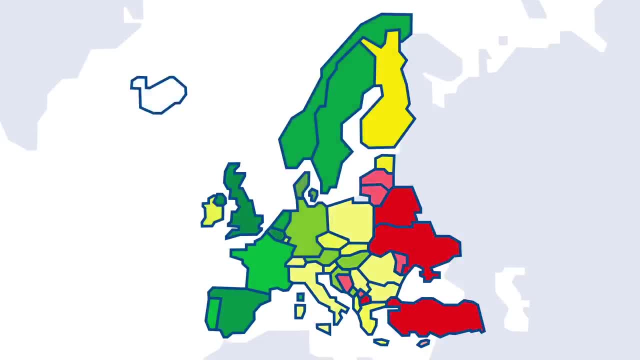 What about social attitudes? Well, this one shows us each country's feelings on LGBTQ plus rights, with a pretty clear East-West split. Economics is probably the easiest to measure, though, with again a fairly clear split when it comes to GDP per capita of European nations. 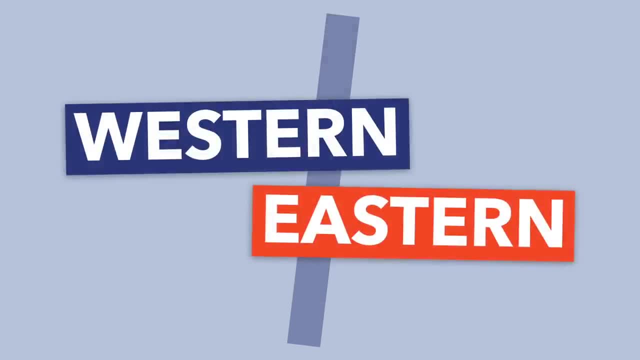 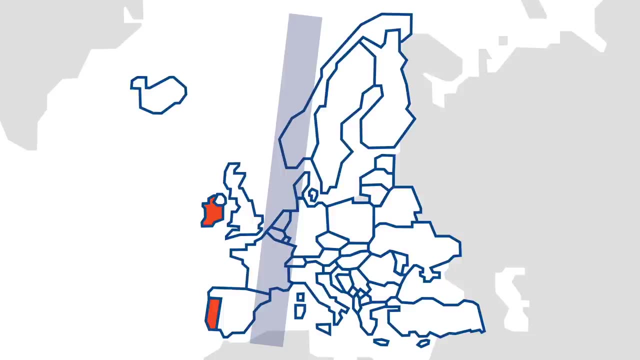 This East-West divide isn't strictly true, though. There are some countries like Portugal and Ireland which are firmly Western geographically but cross the line on some issues socially, like LGBT rights in Ireland, GDP in Portugal and the importance of religion in both. 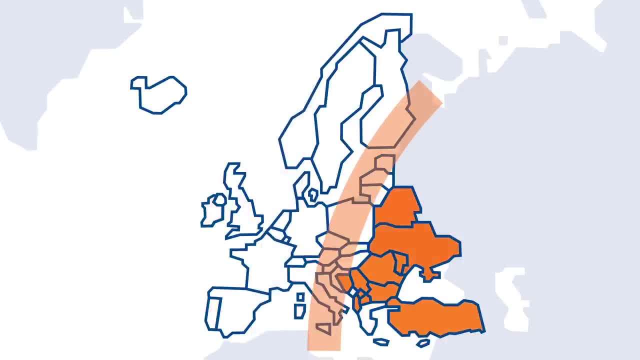 Also, the East clearly isn't a homogenous zone. Some see Russia as a threat, others as a friend. Some are in the Eurozone and others aren't. Some are in Schengen and others aren't. Some think of themselves as more Northern and Nordic. 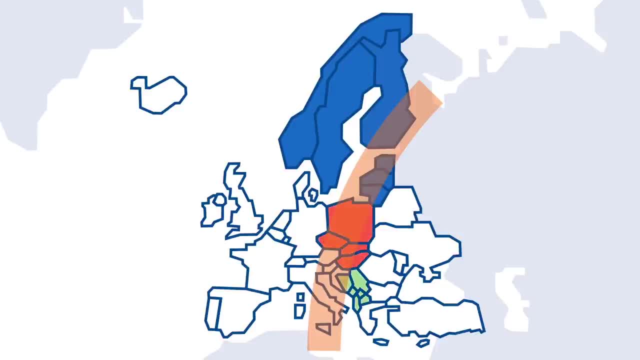 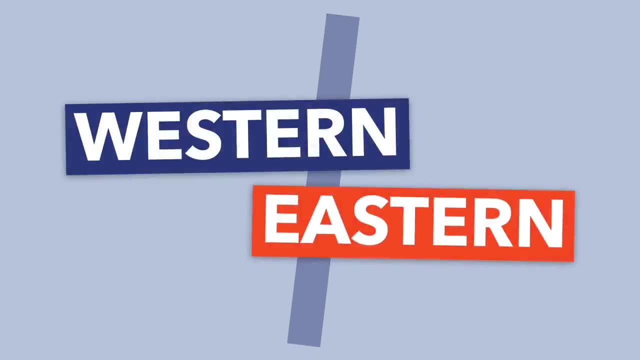 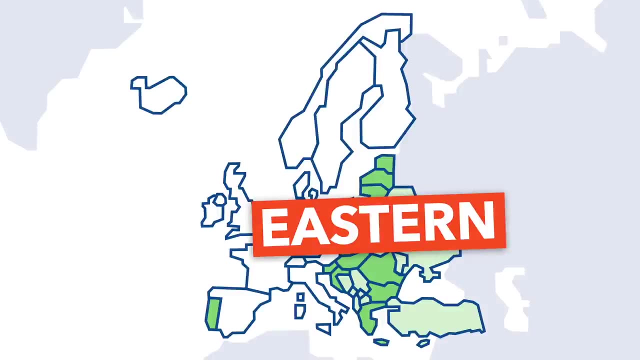 while others have stronger V4 and Balkan identities. That's what makes drawing a line so difficult. Besides straight geography, there's no clear definition of what makes a country feel intuitively Eastern or Western, and when Eastern is often used as a synonym for poorer. 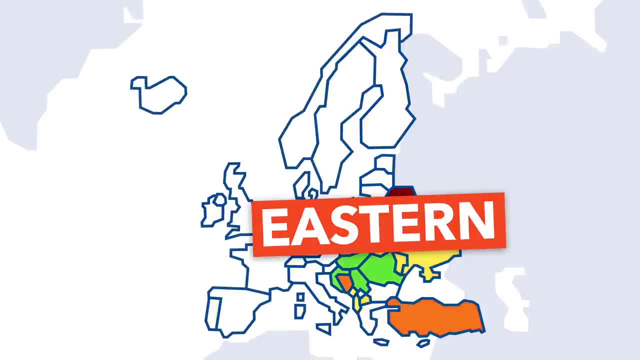 less progressive and less democratic. it's easy to understand why some would want to shrug off the label. In fact, it's that stigma that might explain why only one country was almost unanimously voted Eastern. in the same way, all of these were almost unanimously voted Western. 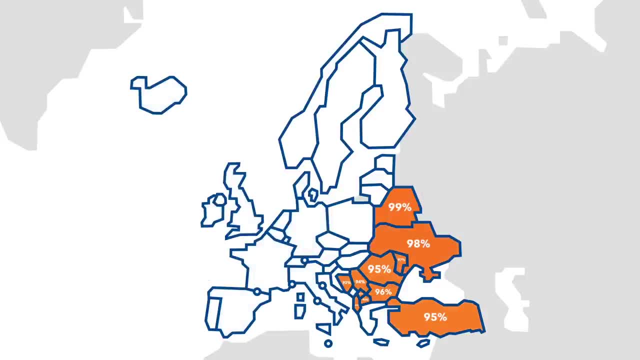 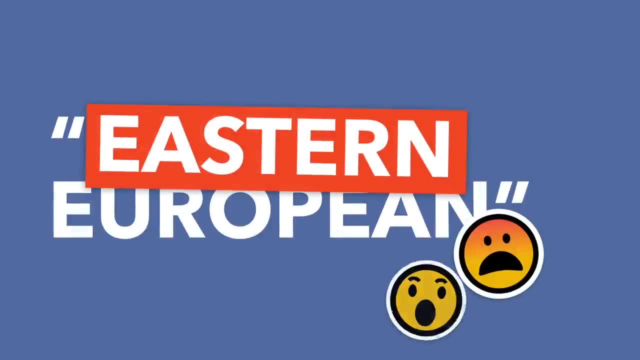 People, especially those living in these countries and areas, are cautious of the Eastern Europe label, and for good reason, with it often hijacked by populists across the continent. In fact, if we look at the countries we've marked as Eastern European thus far, 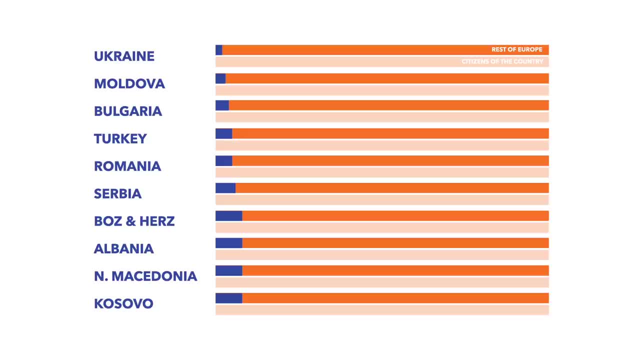 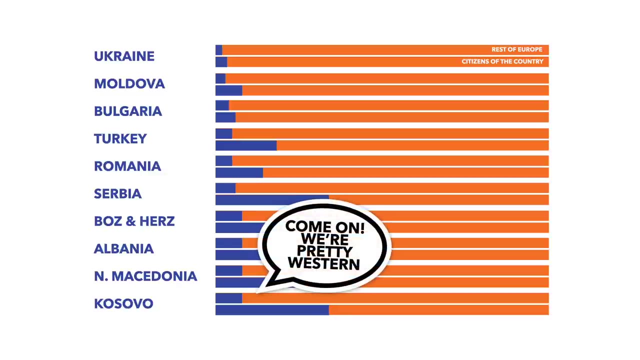 and separate out the people voting from those countries. the average score they receive is consistently more Eastern than the label they give themselves, with every country on this list thinking of themselves as less Eastern than the continent as a whole sees them. That said, let's fill in some gaps and see where the line is drawn by our audience. 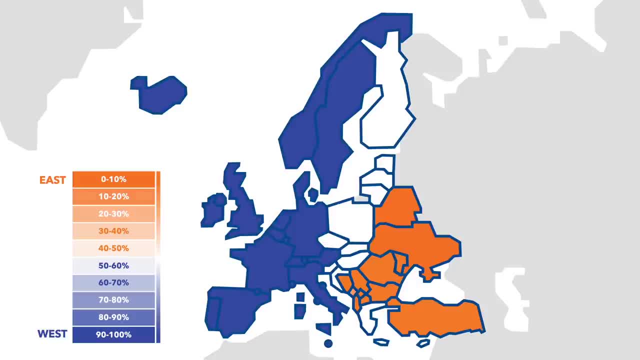 89% of people put Montenegro in the East and 87% put Lithuania and Latvia in the East, slightly more than the 79% Eastern scored by their northern neighbour of Estonia. Both Poland and Hungary came in at 85% Eastern. 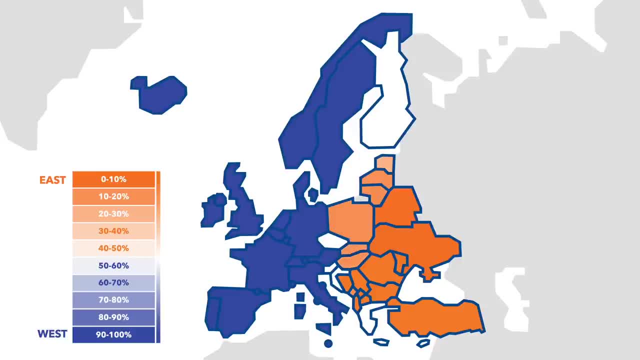 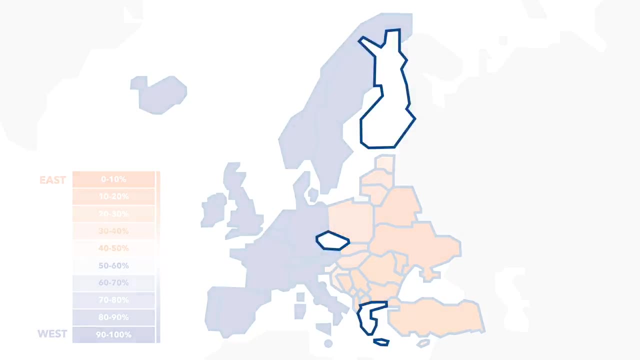 while Slovakia was 84% and similarly named Slovenia was 66%. Despite being significantly further East, Cyprus scored the same as Croatia, with 73% of people, putting them in the East. The very close nations, though, were the Czech Republic, Greece and Finland. 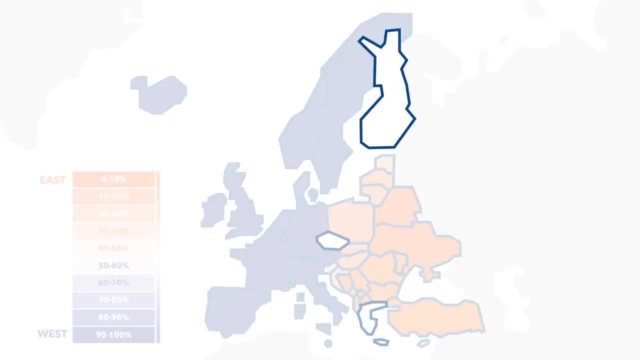 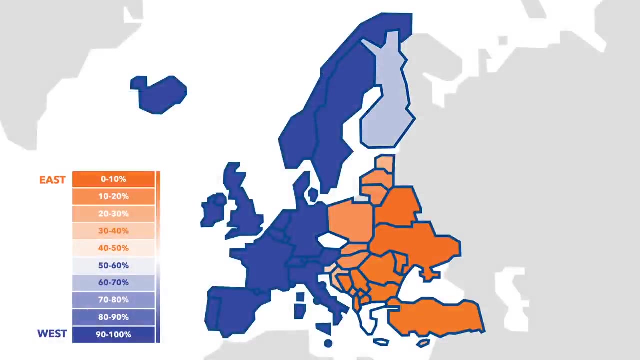 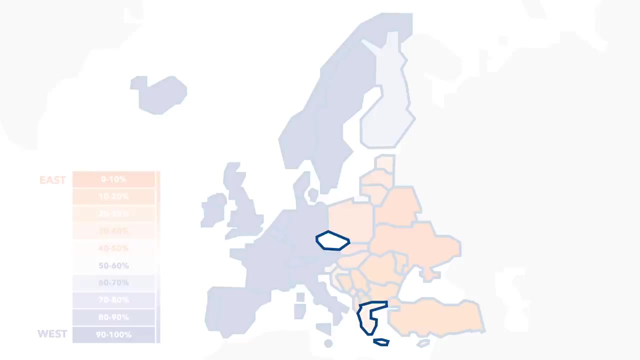 with the latter being the only ones sneaking into the West. Despite being pretty far East geographically, its Nordic connections pulled Finland West in your eyes. Greece and Czechia both slipped the other way, though, with them scoring 58% and 59% Eastern respectively. 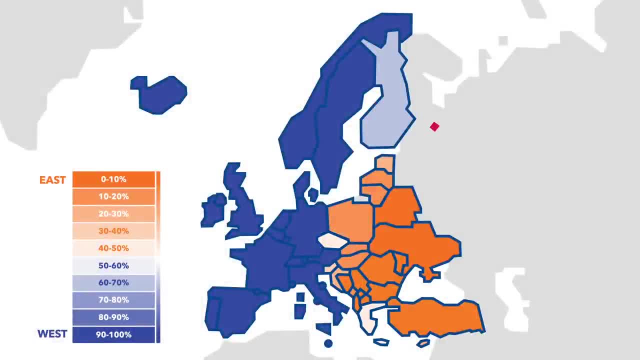 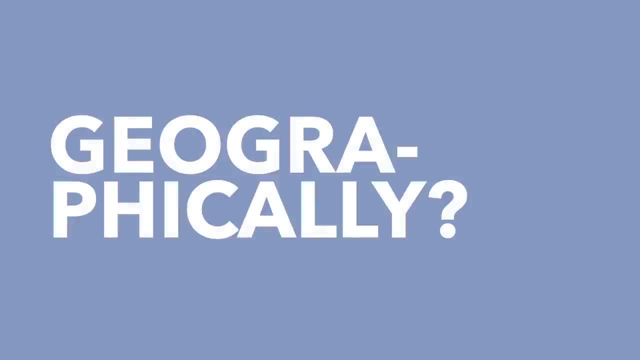 With all of these countries coloured in, then we can finally draw a line dividing the continent based on your votes. But does this line make sense? Well, geographically, kind of, It definitely bends a fair bit to let Finland into the West. 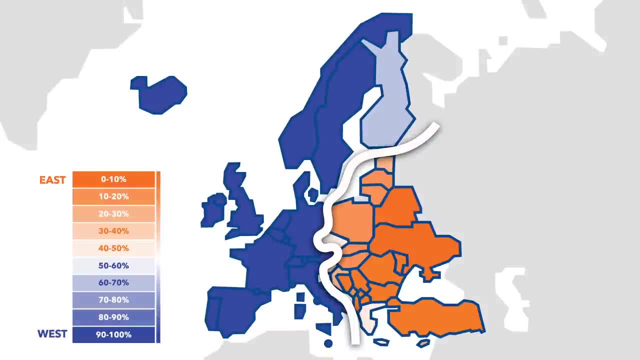 but all in all, it's a pretty geographically accurate line. But what about the factors we mentioned earlier, though? Well, it does seem that the line drawn does fit fairly well with the statistics we discussed earlier, such as GDP per capita, strength of religious convictions. 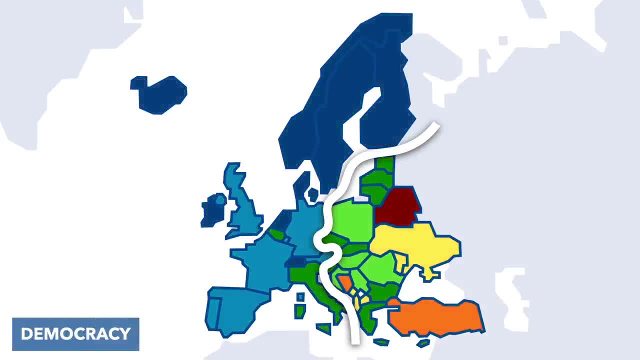 LGBTQ plus rights and democracy. But as we go along, as we discussed earlier, this isn't a straight geographic split on any issue and potentially the label Eastern European isn't even all that useful. Finally, though, as I mentioned at the start, 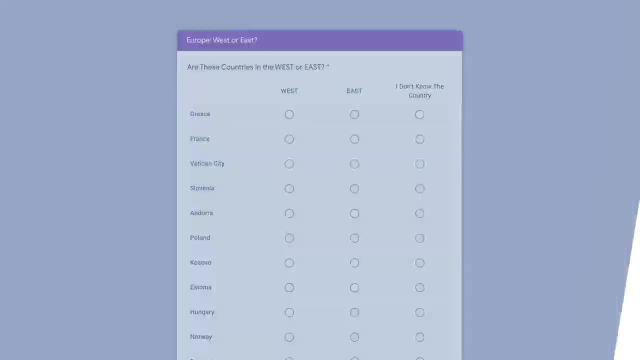 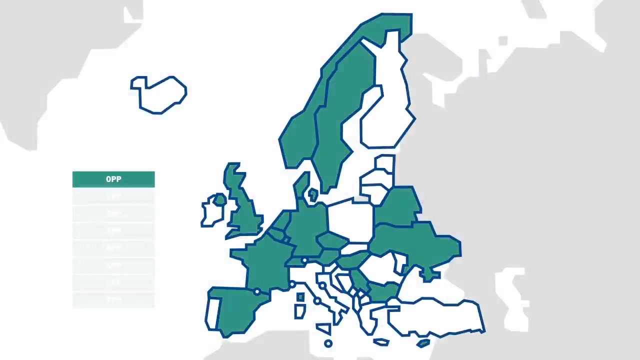 we showed some respondents a map when they were ranking, while others were told not to consult maps. For a lot of countries, seeing the map made no difference. generally those pretty clearly on one side or the other, with the exception of the Czech Republic here. 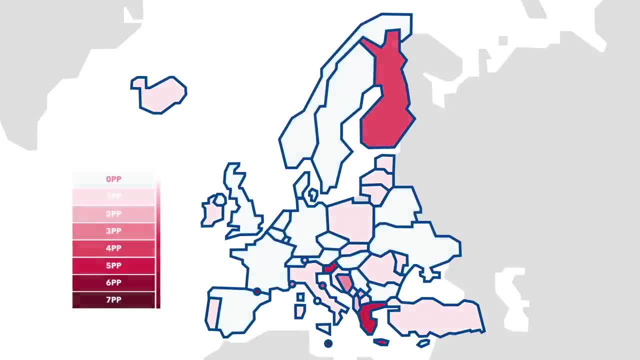 The other countries, though, saw a more notable shift between map viewers and non-map viewers. Now, the ones in blue people rated as more Western once they'd seen the map, and those in orange people thought of as more Eastern when they saw their real geographical location. 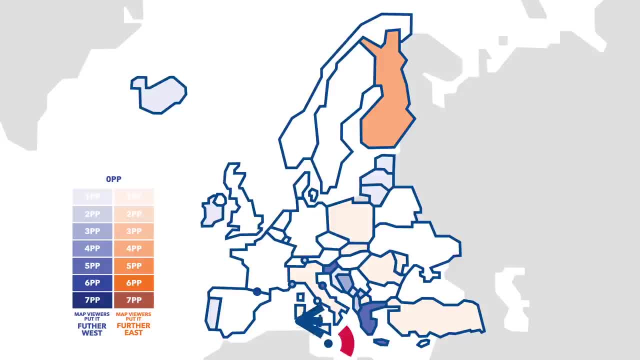 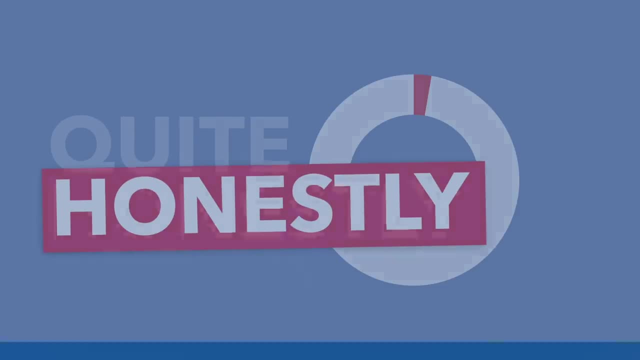 The biggest shift was for Malta, which saw a 7 percentage point shift between those seeing and not seeing the map, with map viewers ranking it as more Western than non-map viewers. Notably, though, 2.7% of respondents very honestly admitted that they didn't know enough about Malta to judge it.